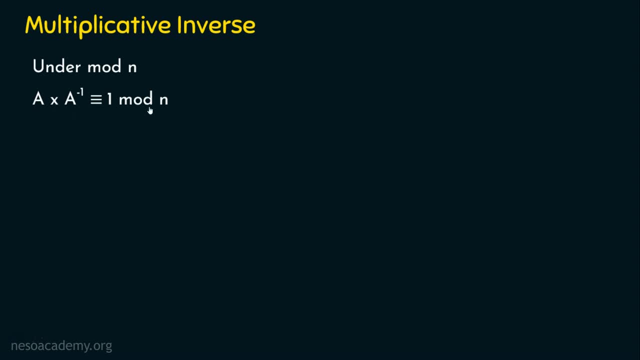 of a and a inverse. when this value is divided by n, we will get the remainder as 1.. So this is the basic idea behind multiplicative inverse. So this is what the idea of multiplicative inverse under modular arithmetic operations. We have already seen this example previously. 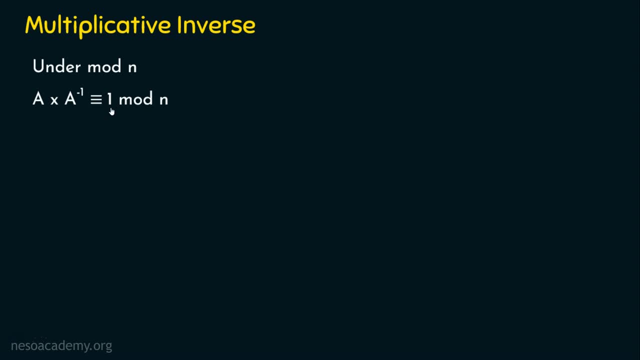 5 is the number 1 by 5 is the multiplicative inverse. So obviously 5 multiplied by 1 by 5 will be 1, isn't it So for the number 5,? always 1 by 5 is the multiplicative inverse. 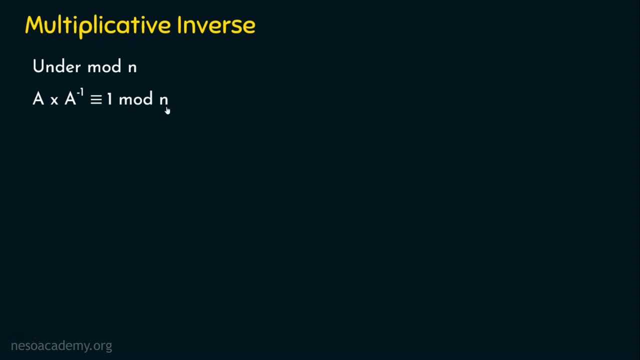 But when you are finding multiplicative inverse under mod n, there cannot be a fixed number. For example, the multiplicative inverse for 2 mod 5 is different and the multiplicative inverse for 2 mod 7 is different. You may be thinking like you are going to find the multiplicative inverse for 2 only. 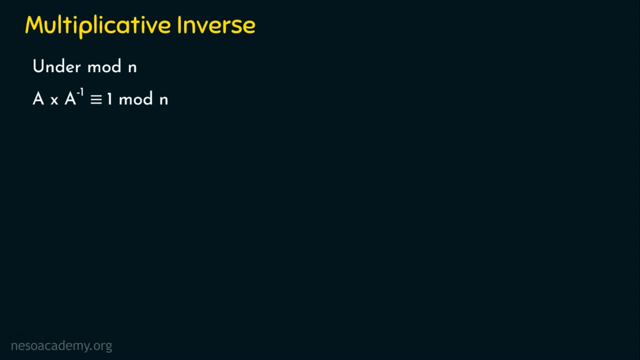 But please note it's not simply 2,, it's 2 mod 5 and 2 mod 7.. So the multiplicative inverse for 2 mod 5 is going to be a different number and the multiplicative inverse for 2 mod 7 may be a different number. 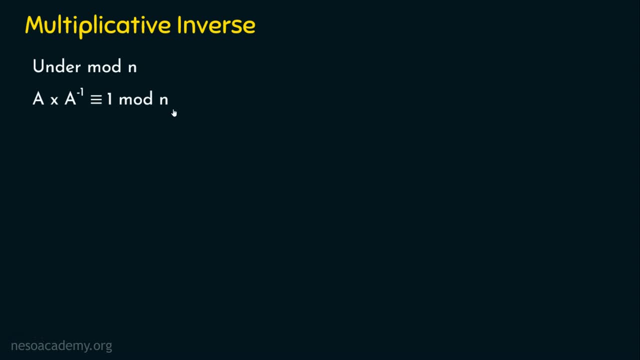 We need to have an understanding on this. Let's understand. Let's understand things clearly now. Let's say there is a number 3.. Now we are going to find the multiplicative inverse of 3. It is 1 by 3, obviously, when it is a normal number. 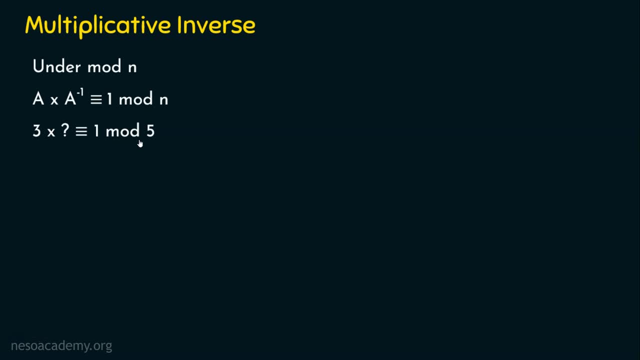 But when modular arithmetic is involved, mod 5, right. So what is the multiplicative inverse for 3 mod 5?? That's the question is actually. So we are required to find the multiplicative inverse of 3 mod 5.. 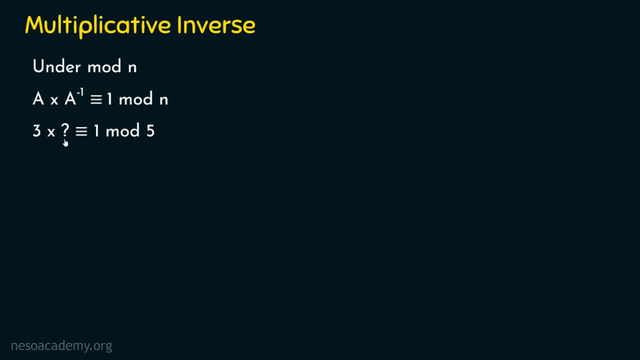 Not simply 3,, it's 3 mod 5.. So what do you mean by this? I already told you: when you have a number, when that number is multiplicative, when it is multiplied by its inverse, we will get 1 as the remainder. when this product is divided by n, 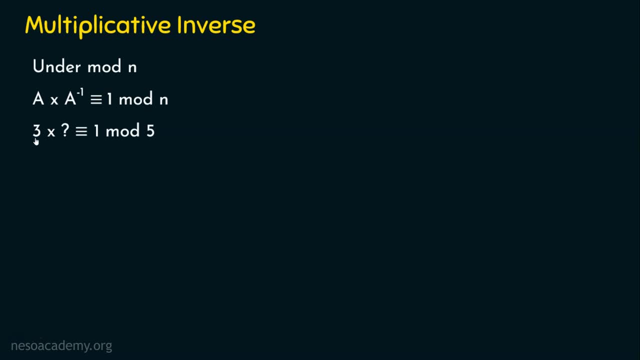 So, similarly, when we have a number here, 3,, when this 3 is multiplied by its inverse, then the whole result, that is, this product when it is divided by 5, we should get 1 as the remainder. Let's try the number 1.. 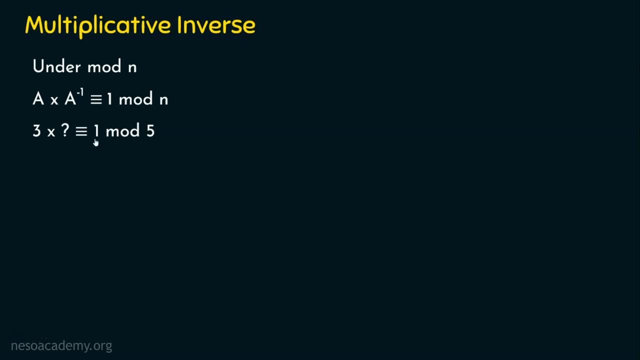 3 into 1 is 3.. So 3, when it is divided by 5, we get 3 as the remainder. So 1 is not the multiplicative inverse for 3.. Let's try with 2.. 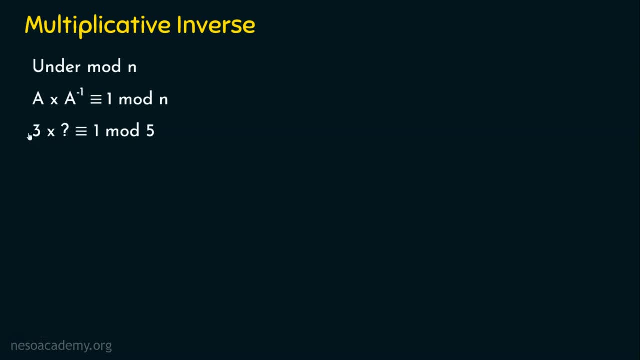 3 into 2.. 3 into 2 is 6.. So this side we have 6.. When 6 is divided by 5, we get 1 as the remainder. So 2 is the multiplicative inverse of 3 mod 5, or 3 is the multiplicative inverse for 2 mod 5.. 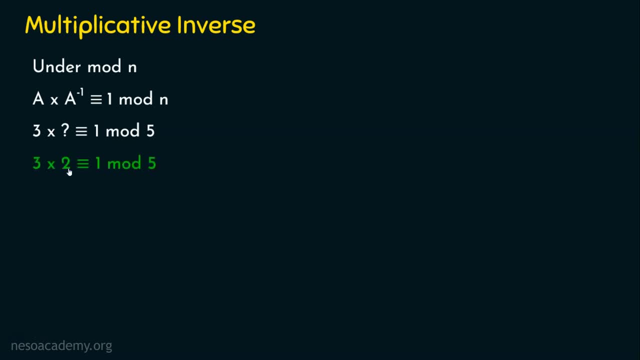 So it's clear that for 3 mod 5, the multiplicative inverse is 2.. Let's say we have a number 2 and we are required to find the multiplicative inverse of 2 mod 11.. So what's the idea? 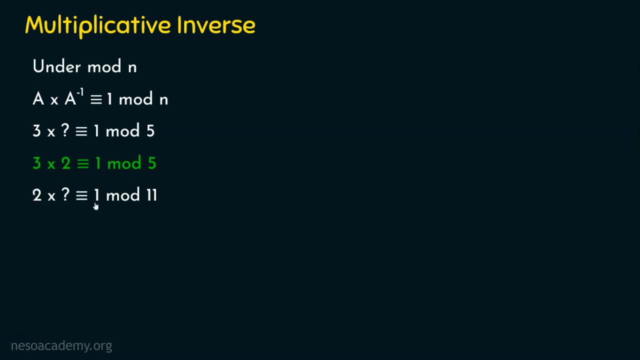 When this side is divided by 11, we should get 1 as the remainder. What is there in this side? It's the product. So 2 is multiplied by which number, We will get 1 as the remainder when this side is divided by 11.. 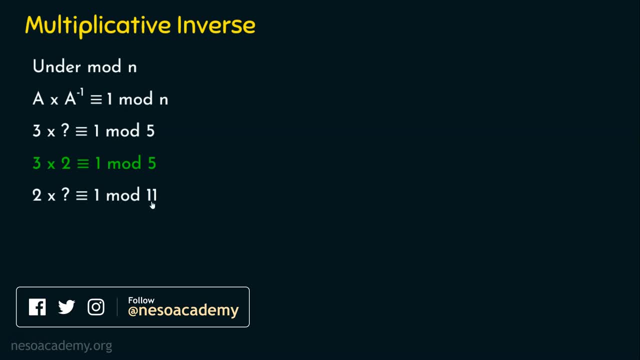 Let's try with 1.. 2 into 1 is 2.. 2, when it is divided by 11, we get 2 only as the remainder. Let's try 2.. 2 into 2 is 4.. 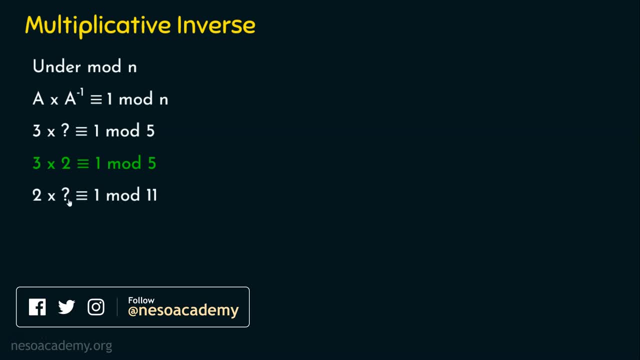 No 2 into 3 is 6.. No 2 into 4 is 8.. No 2 into 5 is 10.. No 2 into 5 is what? 10.. 10, when it is divided by 11,, we get 10 as the remainder, or minus 1.. 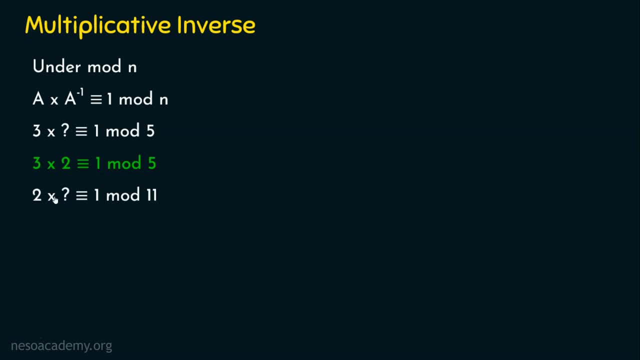 But we need plus 1, right? So let's try with 6.. So 2 into 6 is 12.. 12, when it is divided by 11, we get 1 as the remainder. So the multiplicative inverse of 2 mod 11 is 6.. 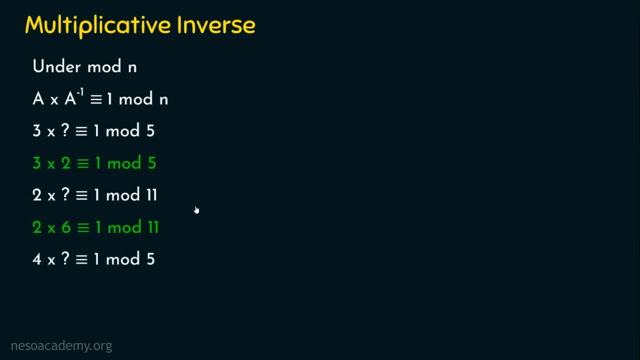 Let's see one more number. 4 is multiplied by what number, We get 1 as the remainder under mod 5.. In other words, what's the multiplicative inverse of 4? Mod 5.. I request you to pause this video for a while. 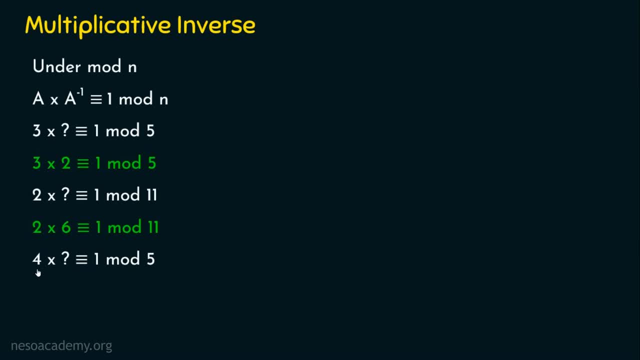 and find out what's the multiplicative inverse for the number 4 mod 5.. I hope you are done. Let me reveal the answer for this. So 4, when it is multiplied by 4, we get 16.. This 16, when it is divided by 5, we get 1 as the remainder. 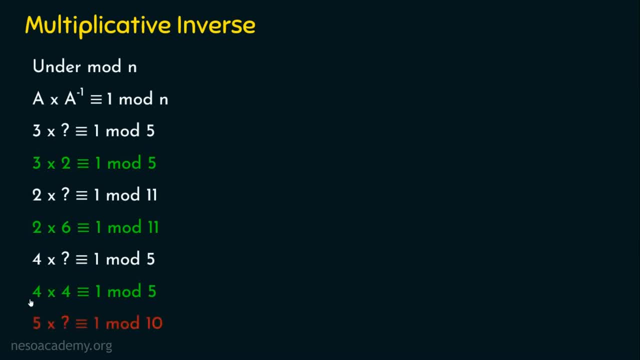 So 4 is the multiplicative inverse for 4 mod 5.. Do we have a multiplicative inverse for this 5,? when it is multiplied by its inverse, we should get 1 as the remainder When this whole side is divided by 10.. 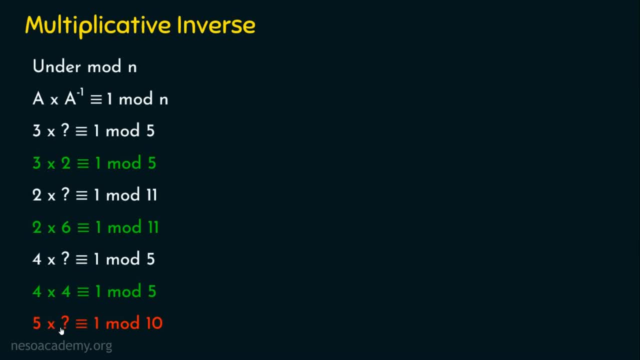 Just try here: 5 into 1.. 5 into 1 is what? 5.. So 5, when it is divided by 10, we get 5 as the remainder. Let's try with 2.. 5 into 2 is 10.. 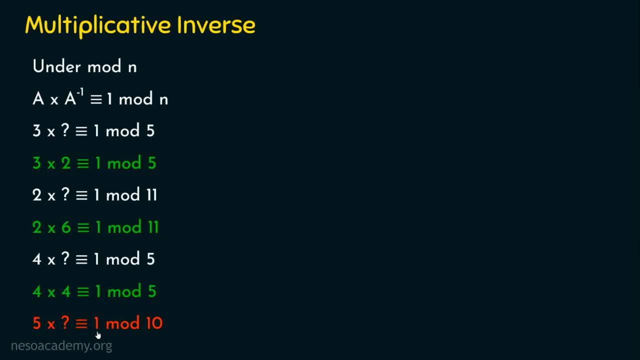 10,. when it is divided by 10, we get 0 as the remainder, not 1.. When you try 3,, we get 5 as the remainder. When you try 4,, you get 0 as the remainder. 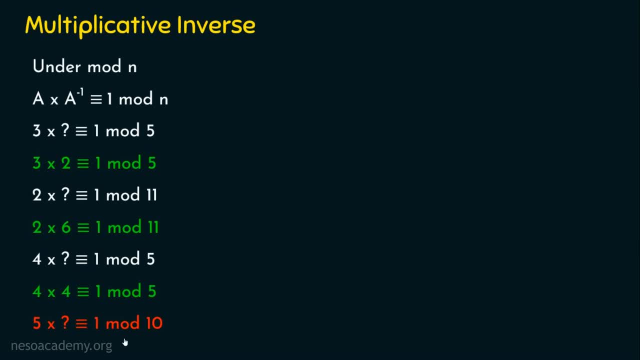 So in this case you will never get a multiplicative inverse if you start applying all the numbers. Do you agree with me? You know why it is so? Because this 5 and 10 are not relatively prime. So multiplicative inverse exists only when this number and this number 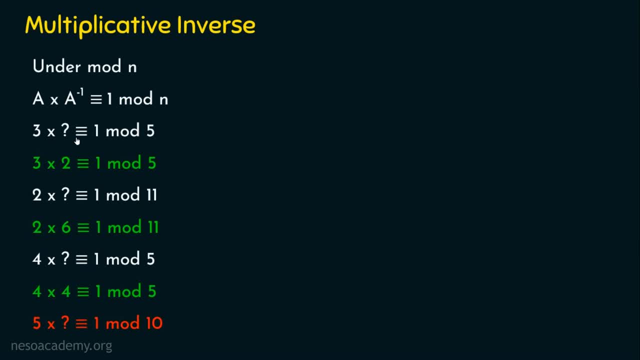 are relatively prime to each other under modular arithmetic. So in this case, 3 and 5 are relatively prime to each other, and that is why we have a multiplicative inverse here. Similarly, when you take this number 2 and 11,- 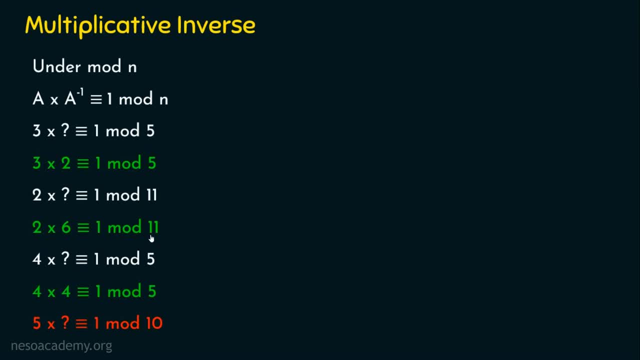 so 2 and 11 are relatively prime to each other. In other words, gcd of 2 and 11 is 1, and that is why there exists a multiplicative inverse for 2 mod 11.. Similarly, there exists a multiplicative inverse for 4 mod 5. 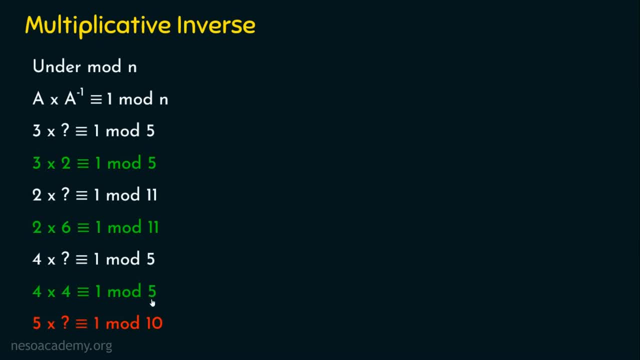 because 4 and 5 are relatively prime to each other. In other words, gcd of 4,5 is 1, and that's why there exists a multiplicative inverse. If the gcd of two different numbers is not 1, then it means they are not relatively prime to each other. 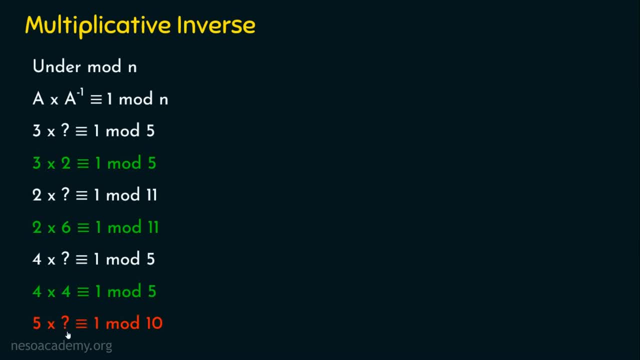 In such cases we will never have a multiplicative inverse. So in this example we can clearly say that 5 mod 10 will not have a multiplicative inverse. You know why? Because 5 and 10 are not relatively prime to each other. 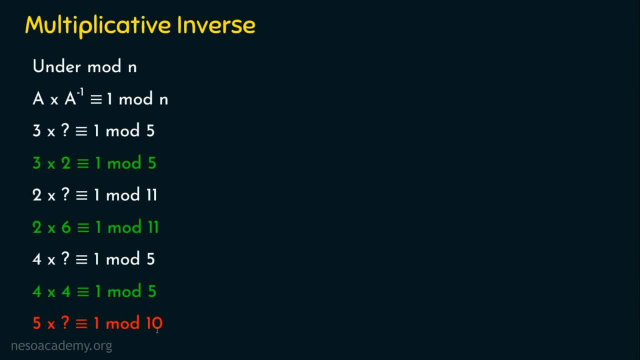 The gcd of 5,10 is 5, and hence we can say that 5 mod 10 does not have a multiplicative inverse. So in the initial part of this lecture I told you the multiplicative inverse of 2 is 1 by 2.. 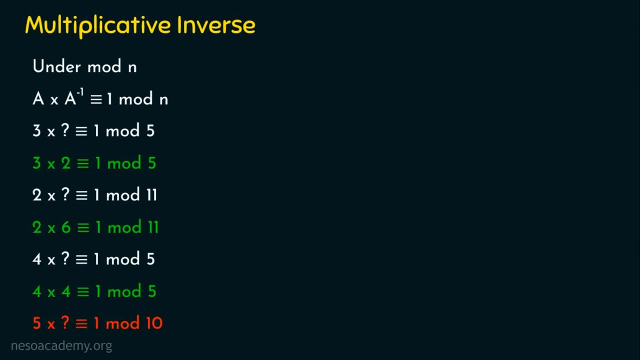 But the multiplicative inverse of 2 mod 5 and the multiplicative inverse of 2 mod 7 are different. That's what I told you. it's not simply 2.. It's 2 mod 5 and 2 mod 7..